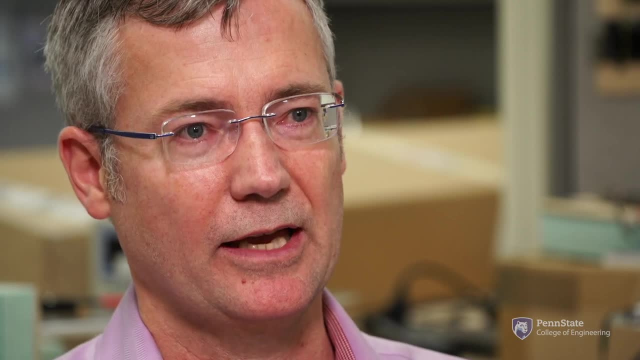 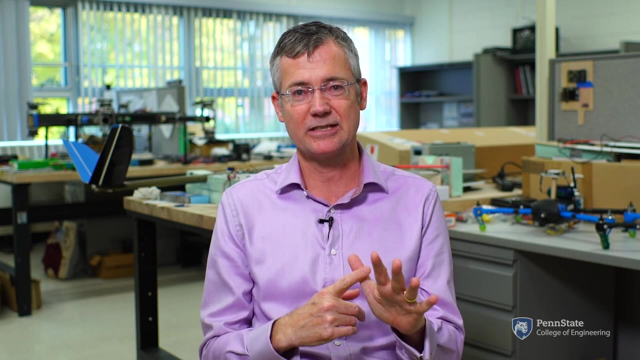 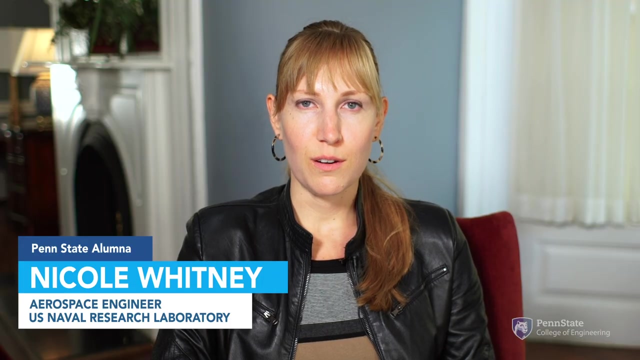 So if you're interested in really big-picture problems and in how the different fields of engineering, like structures or controls or propulsion or aerodynamics or fluid dynamics, all come together in one complicated system, then aerospace engineering is the field for you. You know, it's one thing to sit here on Earth and to look up and think about the things that are above us that we can't see. 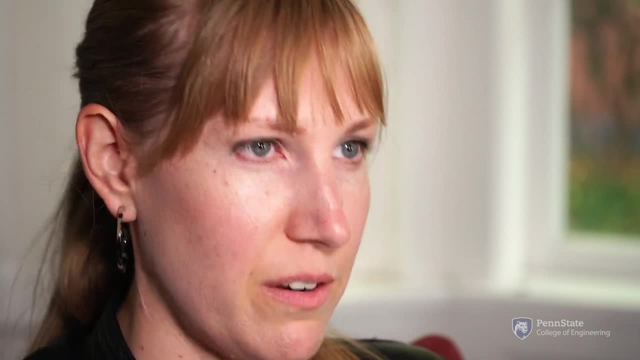 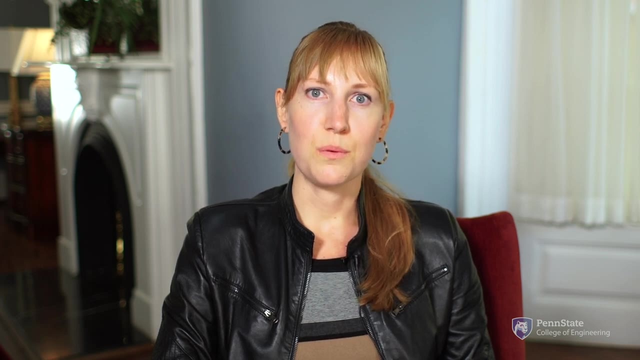 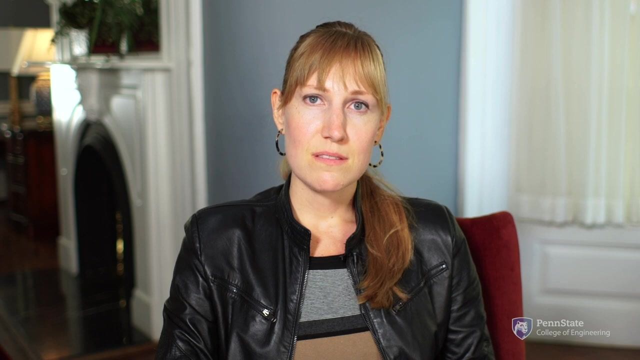 It's another thing to actually be able to figure that out, solve for where these things are, determine where they're going. All of the work that goes into predictions and orbit determinations- we still have this area for improvement. That leaves room for creativity- also extremely interesting. 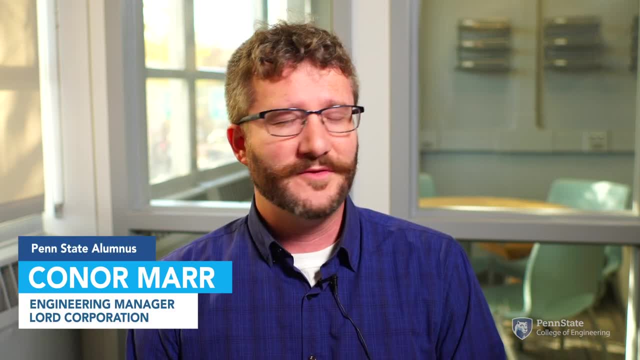 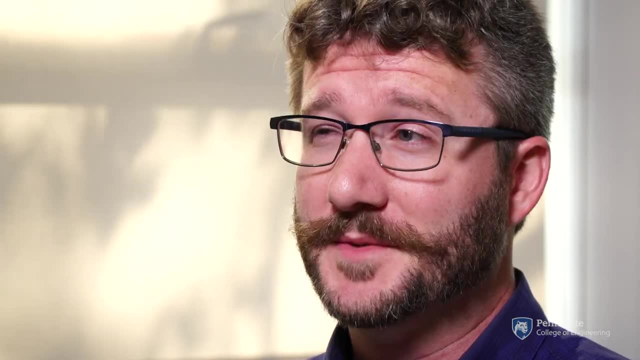 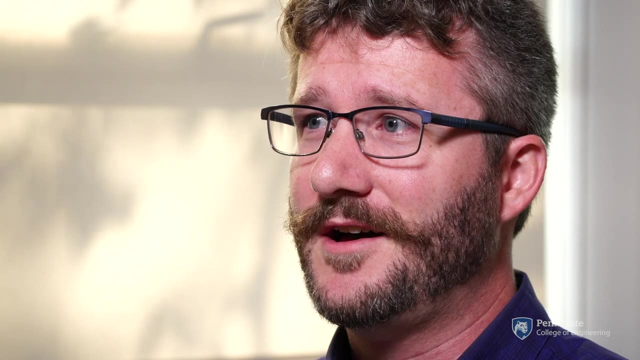 I think my job is very, very exciting. I get to balance so many different things and every day is different. One day I'll be applying my aerospace skills to work on a new design for a helicopter bearing. The next day, I might be working on an oil and gas project where they need some CFD capability. 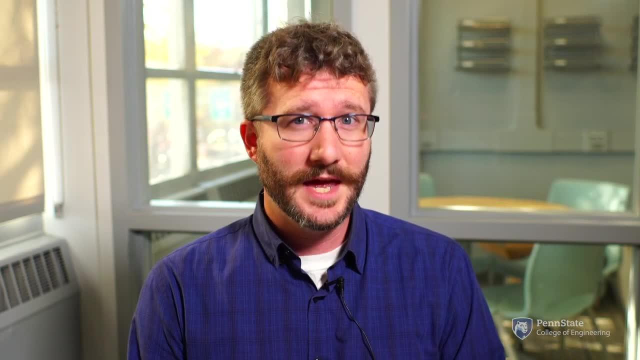 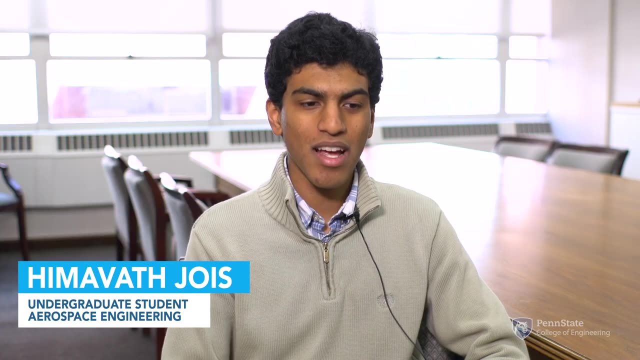 So I love that ability to take ownership of my skills and be able to do that And be able to excite others and solve real problems with them. Aerospace engineering in the modern age has to incorporate so many different things beyond just structural engineering or aerodynamics. 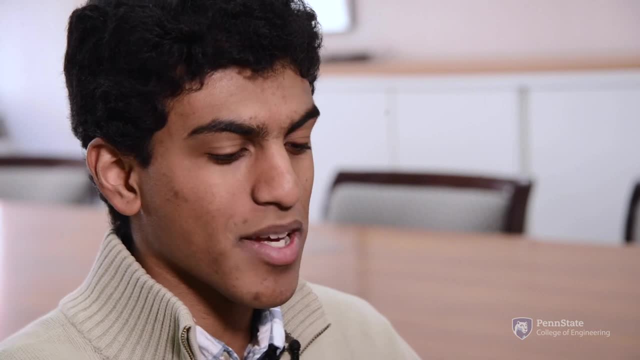 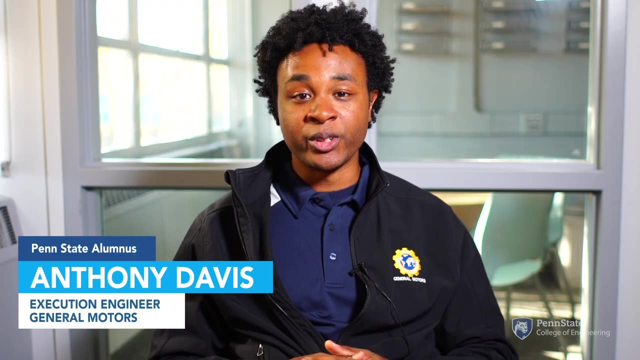 We're able to get this flavor of all the different engineering aspects, from mechanical engineering to computer science, to electrical engineering, to even physics, Aerospace sort of takes all of those different majors and disciplines and throws wings on it or puts it under water and forces it to move. 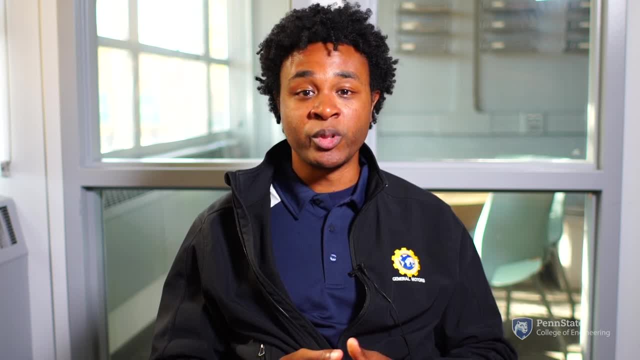 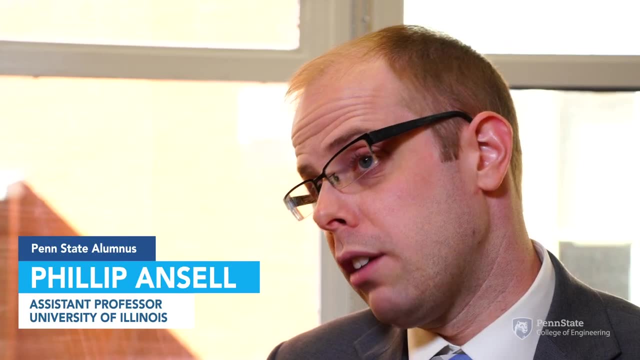 One thing I'd say I love most about being an aerospace engineer is the fact that it's taught me so many different ways to solve problems. Well, it's actually a very exciting time in aerospace The ways that we're kind of looking at taking this new technology that we have with electrically driven propulsion systems. 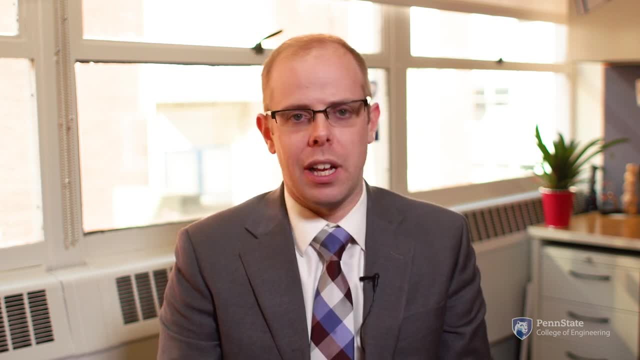 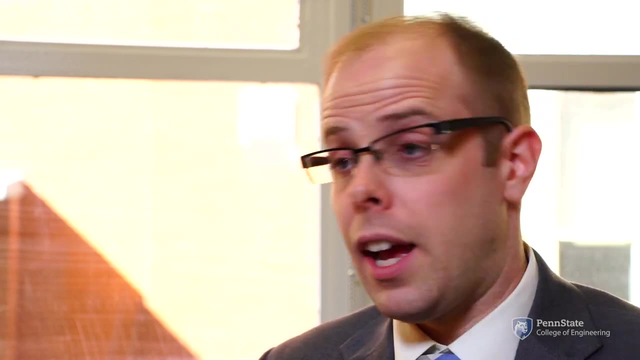 and integrate them into vehicles in novel ways that people haven't thought of. And it's really exciting because now we can make aircraft more efficient, We can make them much more environmentally responsible and actually even cheaper to operate. Across all disciplines, part of our department does material science research.